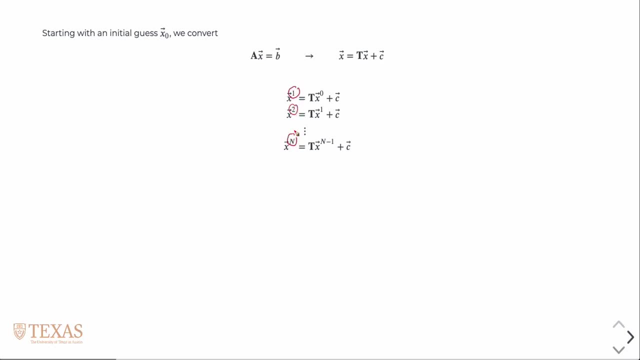 2 and a large n. this is in contrast to the subscript. so in when I have a vector X, I've used the notation to. can you know for the components of the vector to be x 1, x 2? so the subscripts refer to components of the vector. the superscript now refers to the number of. 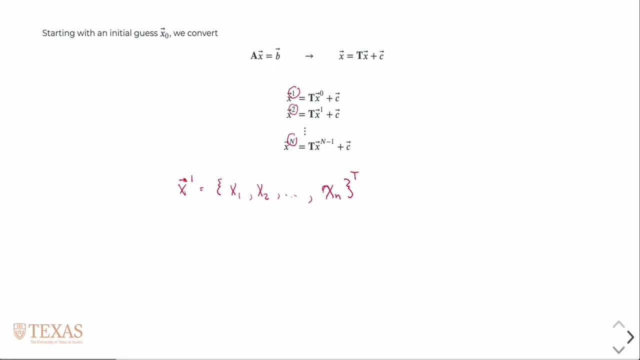 iterations in an iterative cycle or an iterative method. so we'll continue to do this until some convergence criteria is met. there's a number of convergence criteria you can choose. one of them would be where, if X is a vector of, say, the error between iterations, say the error between two and. 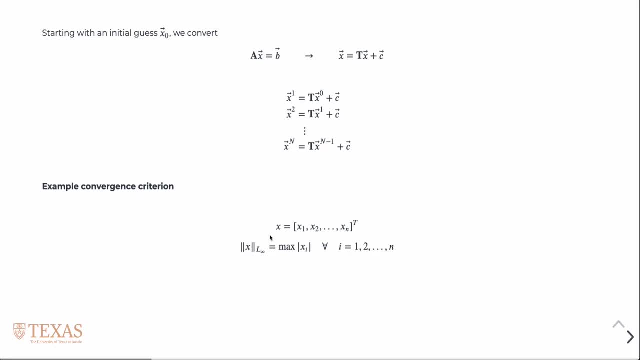 one or n and n minus one, we can compute this L infinity norm. the L infinity norm is simply the maximum absolute value of any single component in the vector. we could then compute that, and if it's below some tolerance we would have the method break out of the iteration cycles. so let's look at an example with numbers. 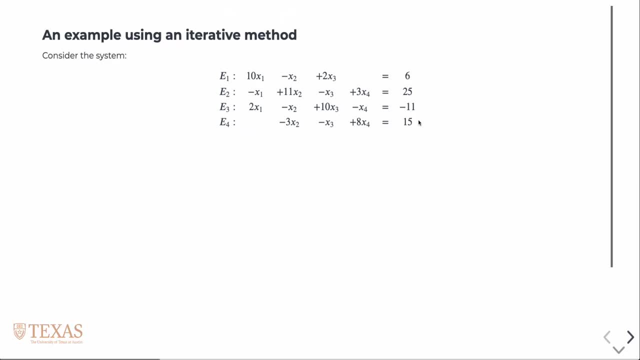 so here we have four equations and written them like this, and what we're going to do is we're going to solve each equation for an attribute that is an X component, and then we'll solve the lattice equation for an X 1, for X 2, and so on, and that's what we have here. I purposely kind of 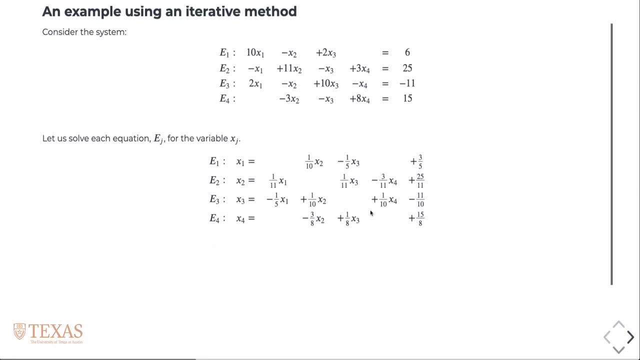 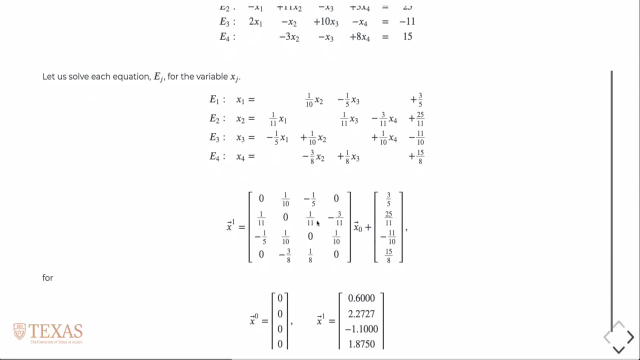 kept the structure of the equations like this. so if we do that and then we write this in matrix form, we have this matrix here. this is this is our tea matrix from before. this is what tea matrix would look like. actually. notice for this particular example, the zeros on the diagonal. then we just stick in an initial guess: x0 for. 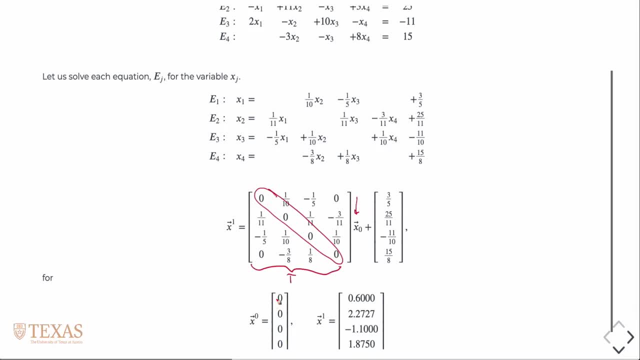 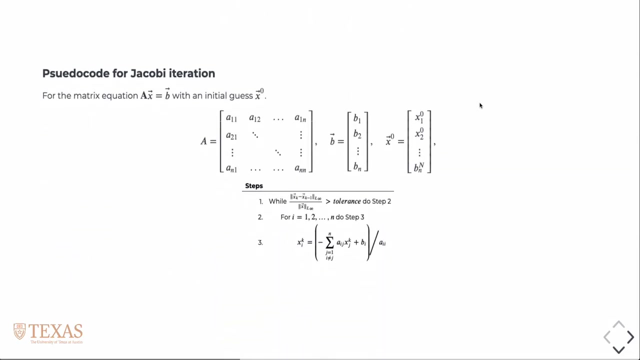 the for the initial guess of x0 equal to zeros, then this is our x1, and we just continue to do this for a number of iterations until the convergence criterion is met, and so this, this is called this process that I just outlined with that example, is called Jacobi iteration, and you'll notice here in the pseudocode that this: 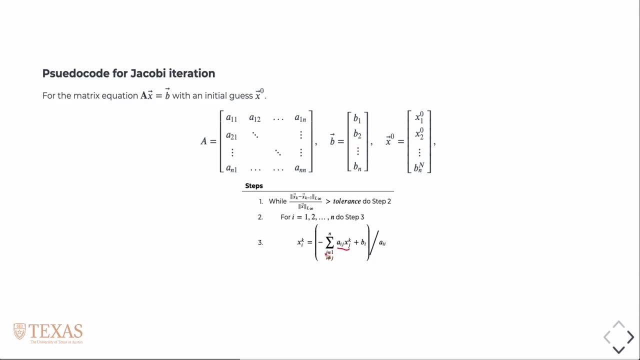 is nothing more than a matrix vector dot product, where we're ignoring the terms on the diagonals. so, in other words, another way to think about that and the way it's written here is that you wouldn't actually compute those terms. but another way to think about it is if you were to just zero out the terms on. 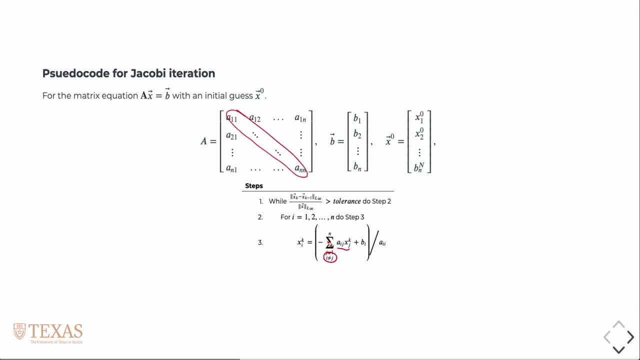 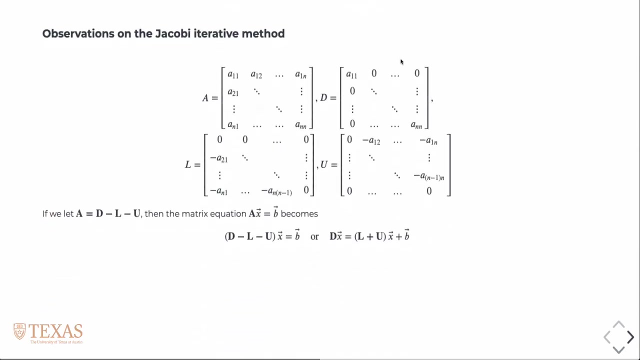 the diagonal and then just do a standard matrix that talk dot, product from the off-diagonal terms, then then you would. that's that's what you would get here, okay, so just some observations. if we take our initial matrix a and we decompose it now, this is not the standard. you know LU, multiplicative decomposition, this is the 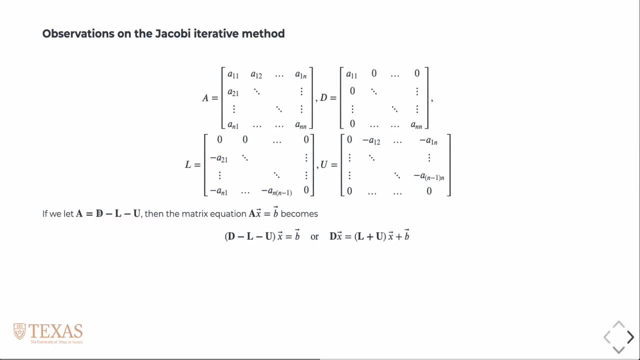 summation of three matrices, right where we have the, the diagonal is just literally the diagonals of a. l is the terms below the diagonals of a, and they've been negated here for good reason, as you'll see as the equations are developed as well as you, is is the. 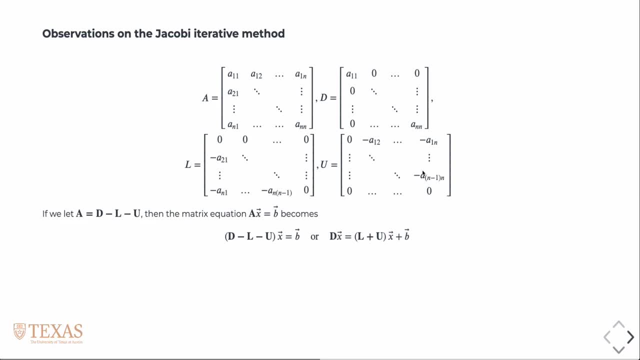 terms above the diagonal of a again having been negated, so that because these terms are are negative, when we take D minus L minus U, then it adds back up to a. So if we plug that into our equation, then we can go ahead and do our separation. 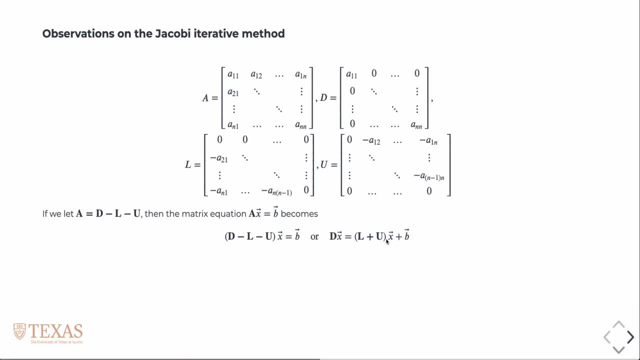 moving the L and U term to the right-hand side of the equation. Then we have this equation here And finally then the solution to that is just the inverse of D, And of course the inverse of a matrix is just one over the diagonal. 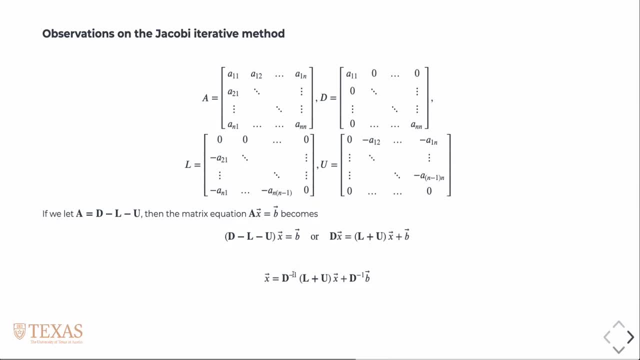 So that's something that's easy to compute. You don't actually have to do any kind of Gaussian elimination or anything there to compute that. But so this would be the matrix form of the Gauss-Seidel iteration, And again just plugging in then the values for K right. 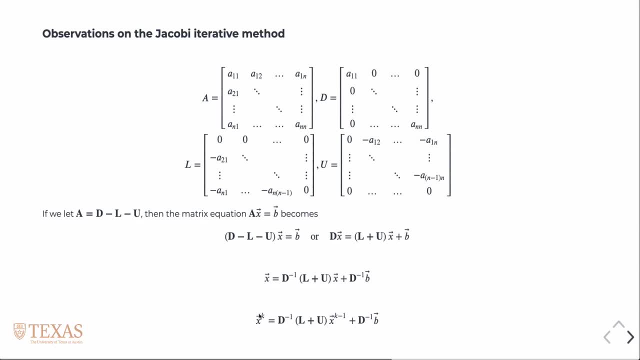 In this case, you know, the superscripted values again correspond to the iteration. So the value at K would be updated with the value at K minus 1.. So you know one thing about If we think, If we think about the Gaussian. 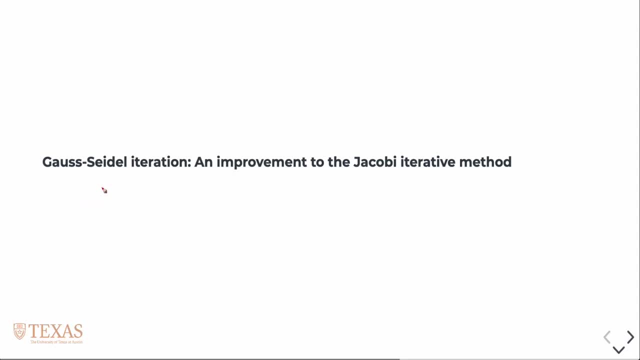 I'm sorry, the Jacobi iteration method. we have this for loop, where we're basically looping over the rows of the matrix. So for I is equal to 1,, 2, to N, where N is the rows in the matrix. 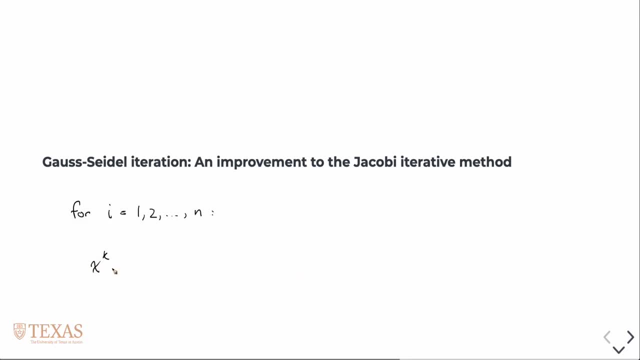 Then we're computing X at K And I'm going to write it in component form, right? So it's XI is equal to the sum. So it's XI is equal to the sum over J. Remember, in the Jacobi we say I not equal to J, right? 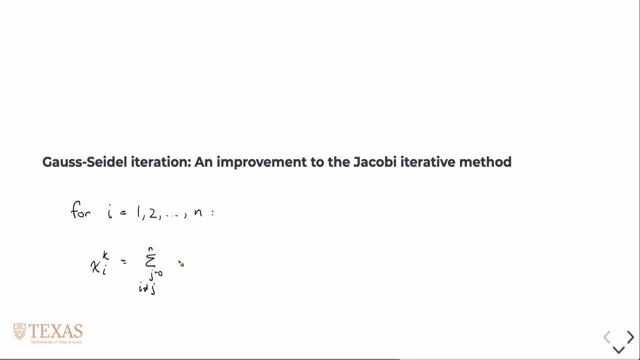 Where J goes from 0 to N, AIJXJ plus, and I'll just say in this case CI, And here we have. this is K minus 1, okay, Okay, But for all I greater than 0, right. 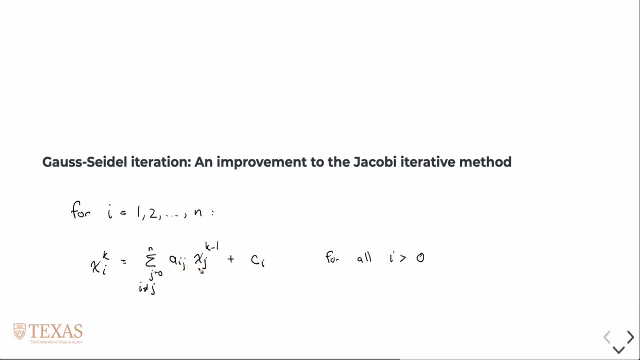 So, once we've passed the first row of the matrix, then the X at K, for that is actually a known value, And so what we'll do is we'll split this summation into two pieces, right, So we're going to not do this anymore, because we're going to split it into two pieces. 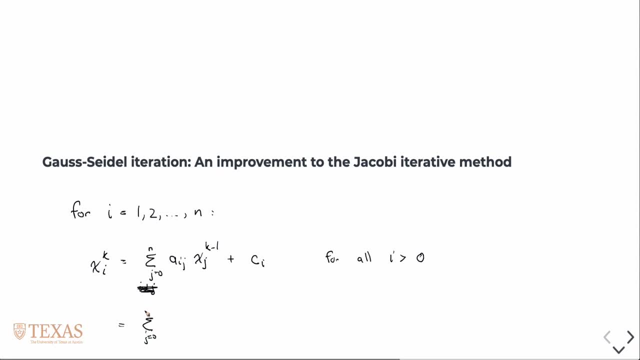 And the first. we're going to go from J equals to 0, to I minus 1.. And we're going to compute AIJXJ, except this time we're going to use the current value because it's already been updated, right. 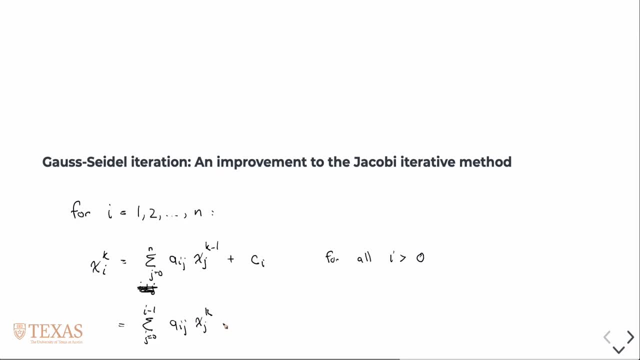 So we're going to use the current value of K, plus, for the ones we don't know, I, plus 1 to N, AIJXJ, And then for these we don't have the current value for K, So we'll just use 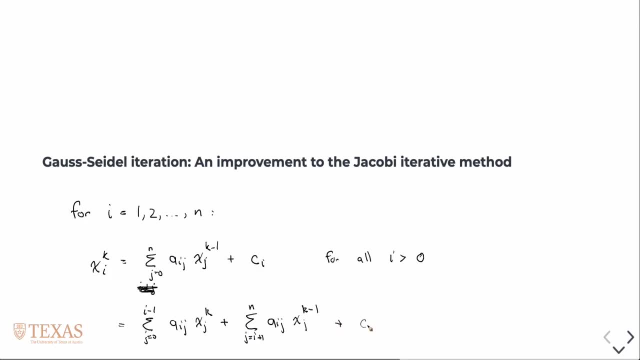 K minus 1, like before, plus CI, And so this process of using the current value. after you've done a few iterations and computed XI of K for the rows above, then we'll use those current values. Otherwise we'll use the old values plus the constant there on the end. 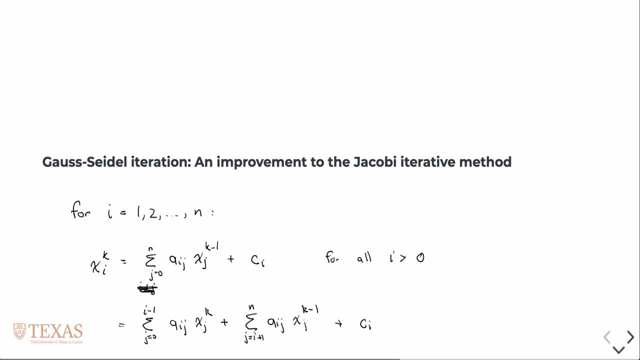 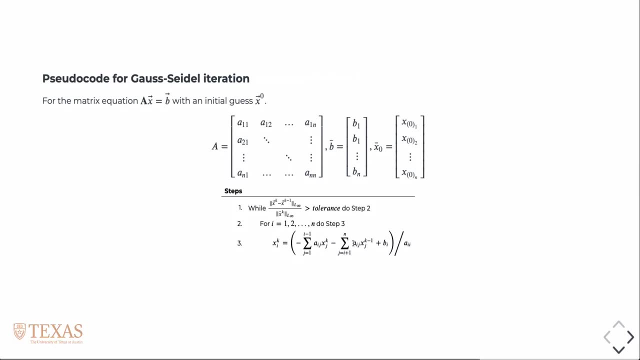 So this process is called Gauss-Seidel elimination And the pseudocode for that is basically just what I wrote there. Again, we're just splitting the summation from 1 to I minus 1 and I plus 1 to N, And using the new value where we can and the old value where we can't. 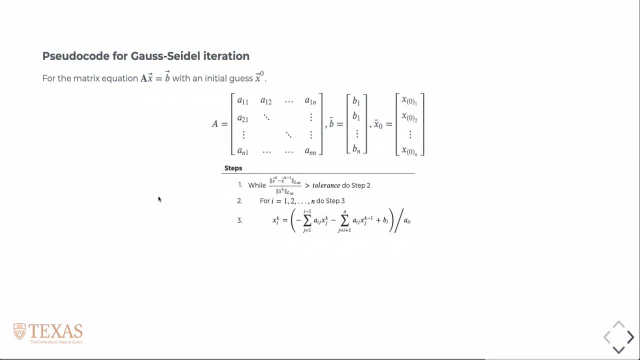 So this process is called Gauss-Seidel iteration And we're going to skip the derivation here. But the matrix, The matrix form of that, looks like this, And I should have mentioned this earlier: There is a necessary and sufficient condition for N minus L. 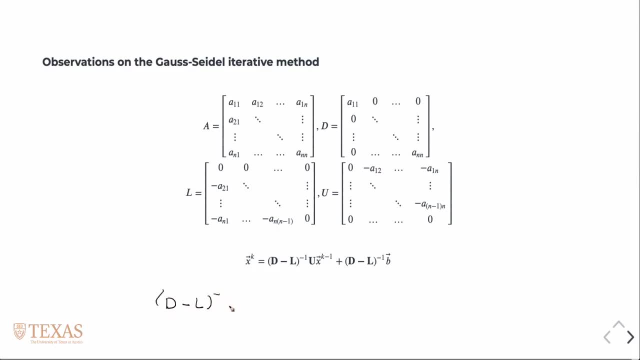 For N minus L to be invertible, for its inverse to exist, then the diagonals cannot equal to 0.. This would be the same in the Jacobi case, where we needed to compute D inverse. Same condition: The diagonals cannot be 0.. 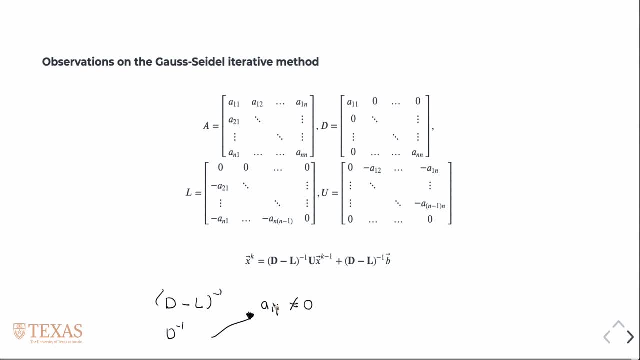 What's not included in the pseudocode is the possibility that you may need to swap rows to ensure, before you start the iteration, to ensure that there are no 0s on the diagonal. So let's quickly talk about the convergence of these methods And in order to do that, we have to introduce a definition, that is, the spectral radius. 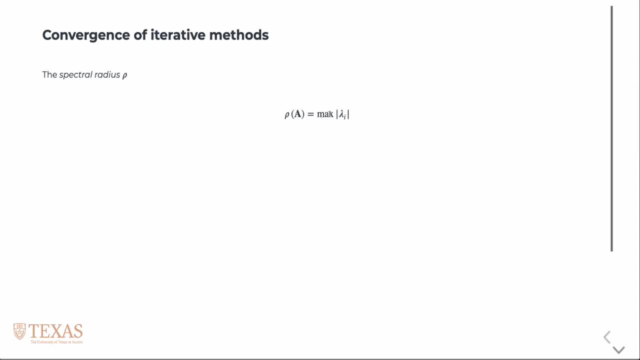 So this, What the spectral radius is, is the maximum absolute value of one of the eigenvalues of a matrix. Now, if you don't know what an eigenvalue of a matrix is, we'll cover it later, But for now we'll just move on. 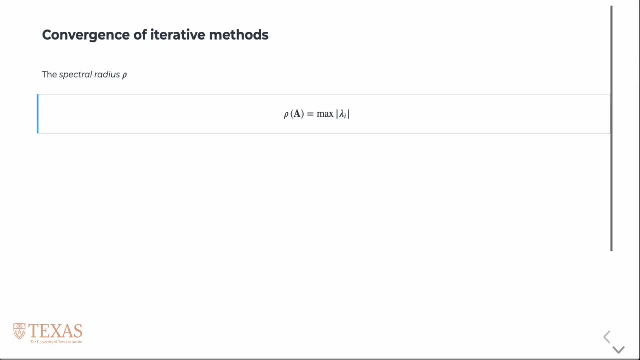 It's a concept from linear algebra, So So what we're going to say is that if the spectral radius is less than 1, then there's an identity that says that For a matrix, A I minus A, inverse is equal to this thing. 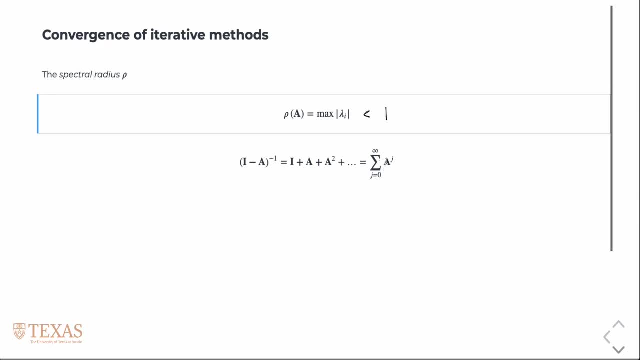 Basically the sum of the powers of the matrix A. So we're just going to hold on to that identity. Again, this is true if the spectral radius is less than 1. The inverse exists and It's equal to that. So if we then look at our